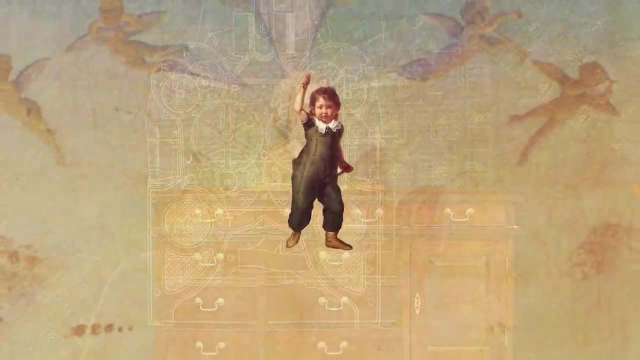 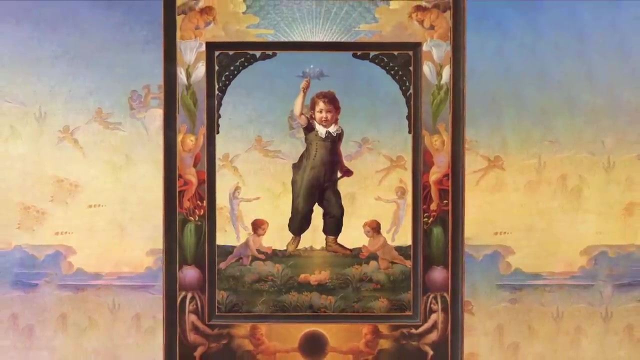 Rousseau emphasises the child, the original rebel, the representative of everything that is pure, unschooled and outside of adult discipline. It is the seat of creativity and genius. For the first time in Western history, glamour is directed not at the attainment of reason. 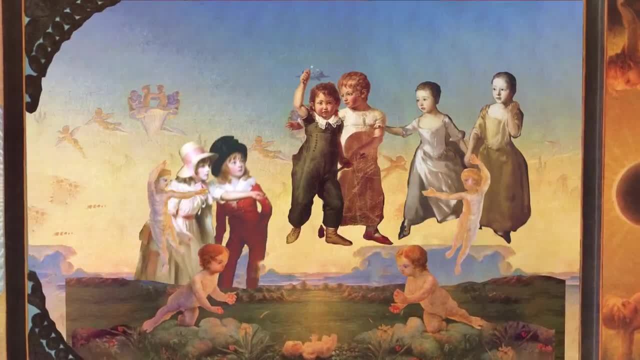 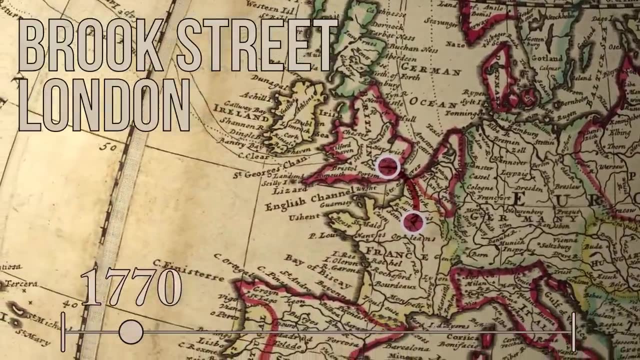 and adult self-discipline. It is directed at the achievement of the right to be a child at self-control, but at the freedom from tradition and the natural innocence and sweetness of the child. Brook Street, London, August 1770.. A precocious 17-year-old poet called Thomas Chatterton downs 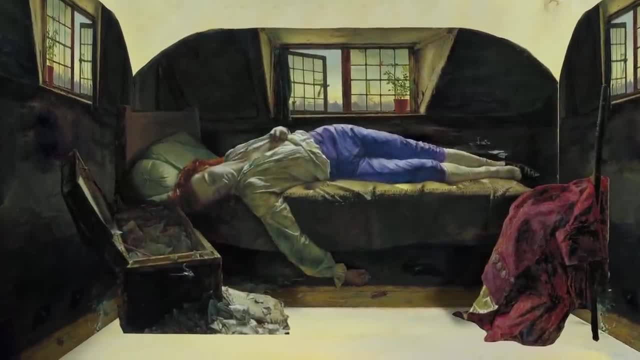 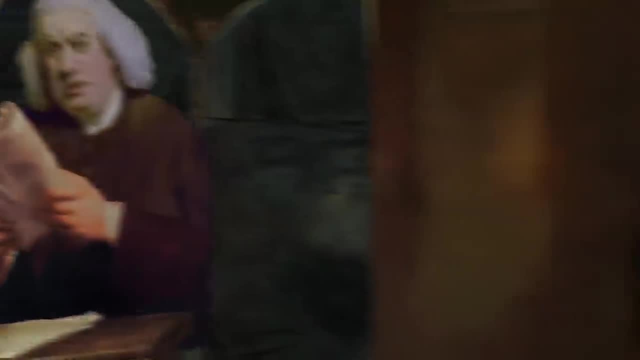 some arsenic and ends his life in a tiny attic apartment. He kills himself because no one wants to publish his poetry, which is concerned with beauty and wisdom, and because his uncomprehending family are applying pressure for him to become a lawyer. A cult soon grows up around the 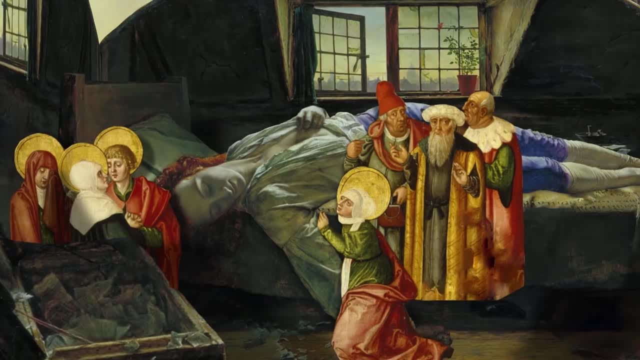 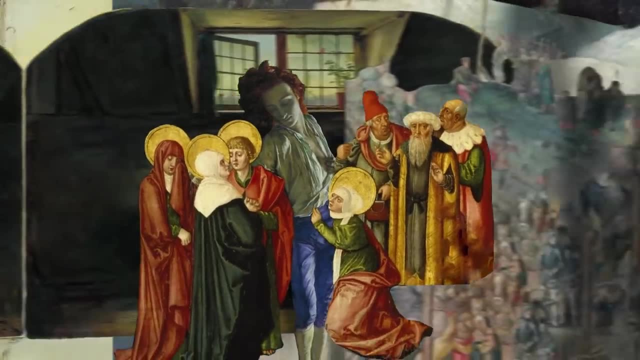 young, beautiful poet. He is a man of his word. He is a man of his word. He is a man of his words. He is a poet with shoulder-length chestnut hair. He becomes an emblem of something that will become very important for romantics – the idea of the sensitive, doomed person. often, 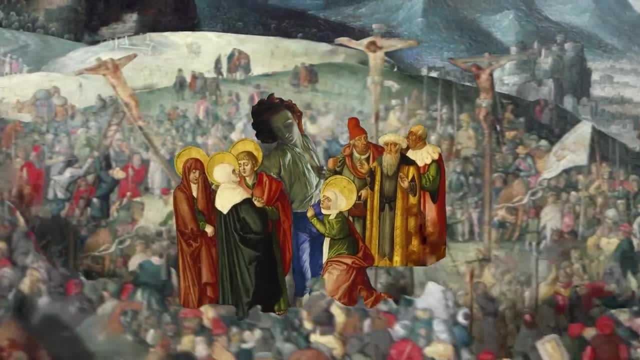 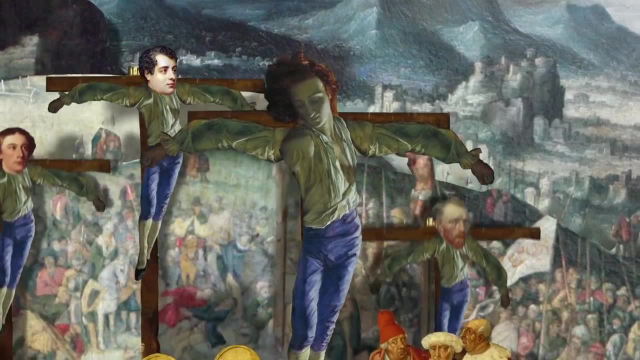 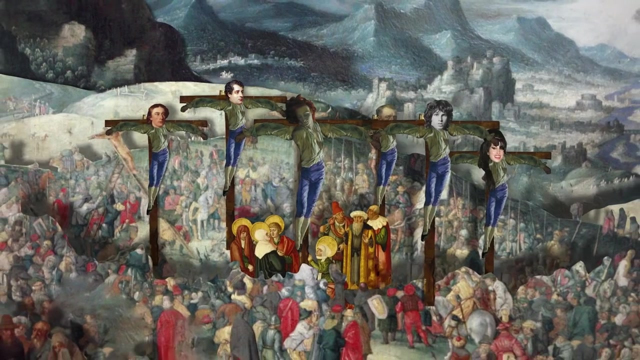 an artist rejected by a cruel, vulgar world. Chatterton stands at the head of a long line of romantic heroes that will stretch from Byron to Keats to Van Gogh and eventually, all the way to Jim Morrison and Amy Winehouse. Romanticism borrows from Christianity. The romantic hero is a secularised Christ-like. 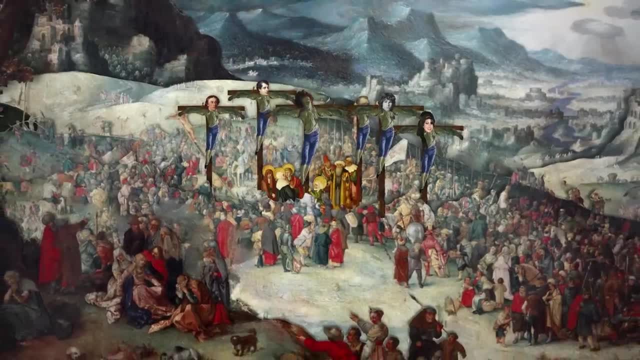 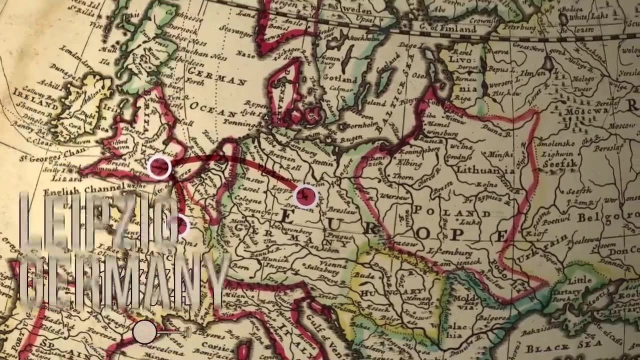 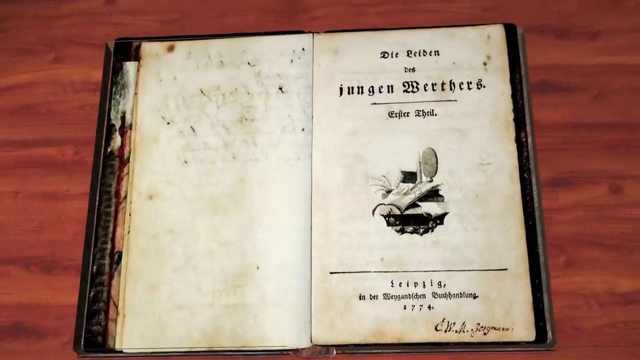 figure the loser, who is in truth deeply noble in the eyes of the few who understand. Leipzig, Germany, 1774.. The German author Goethe publishes the quintessential romantic love story, The Sorrows of Young Werther. It tells the story of a passionate doomed. love affair between a young poet called Werther and a beautiful, clever young woman called Charlotte. Unfortunately for Werther, Charlotte is married. so the love is impossible from the very start. But the love is not impossible. The love is not impossible from the very start. 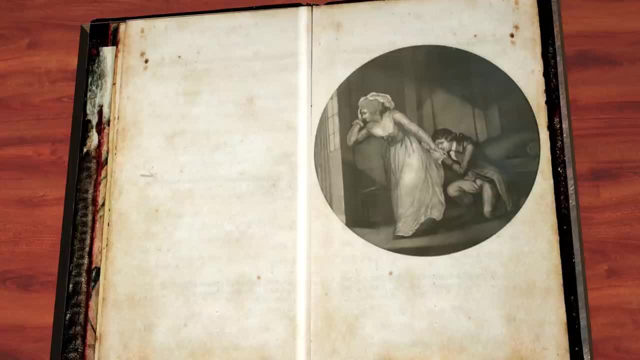 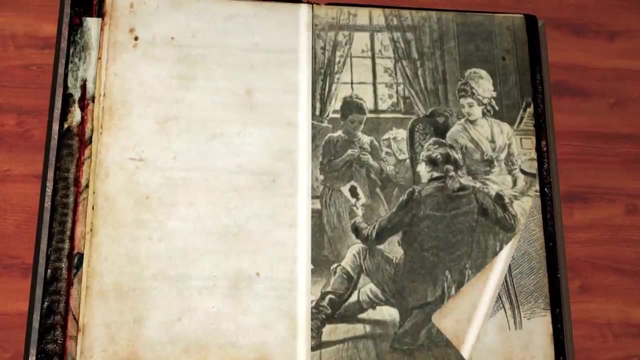 but that doesn't stop Werther, a dreamy, impractical young man who loves the arts above all else. Like Chatterton, Werther is under pressure to have a sensible career and join bourgeois life, but he can think of only one thing – the impulses of his heart. Eventually, 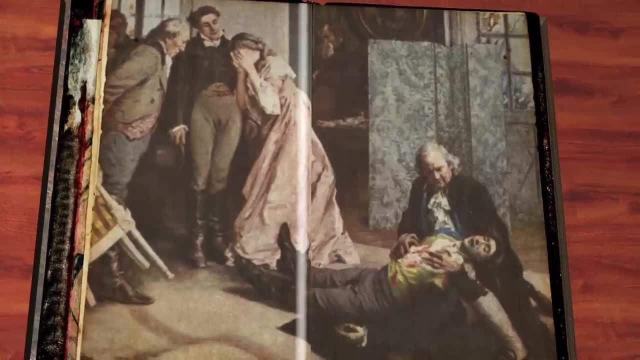 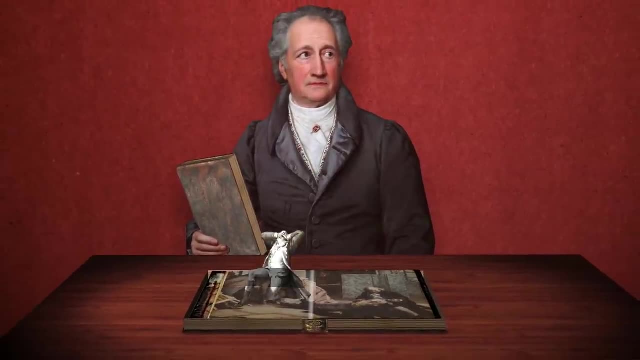 Werther can't take it any more and kills himself. But rather than condemning him as a lunatic and a hothead, Goethe, one of the founding fathers of romanticism, directs all our sympathies towards Werther. We're supposed to be on his side, admiring his passionate 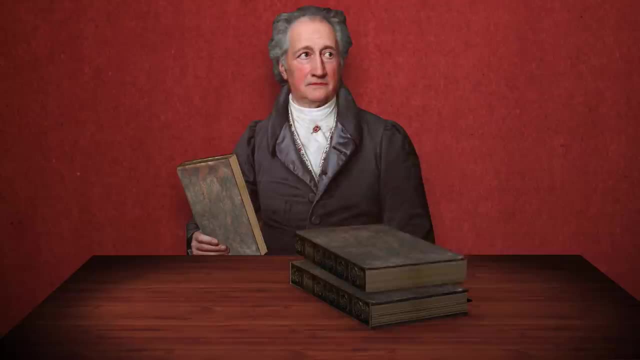 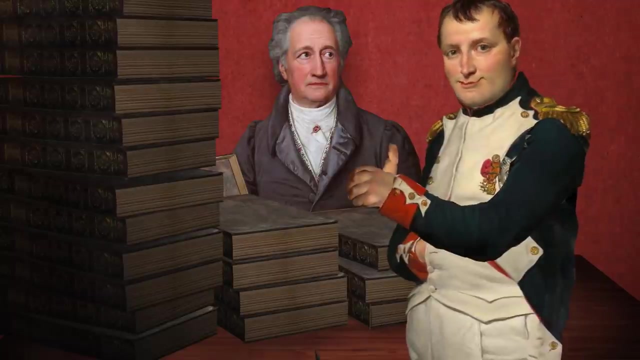 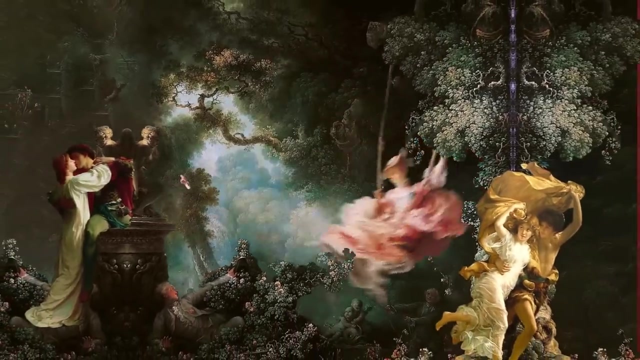 lovely, impractical attitude to love. The book becomes the most popular novel of a generation – three million copies are printed. Napoleon declares it the greatest work of European literature, and it dramatically changes how many people think of love, privileging dramatic outpourings of feeling over more traditional rational concerns for class, lineage and money. 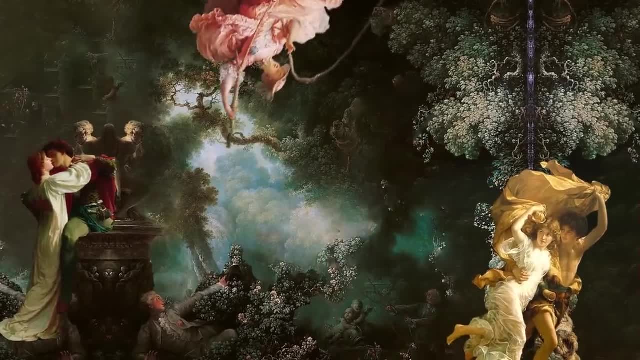 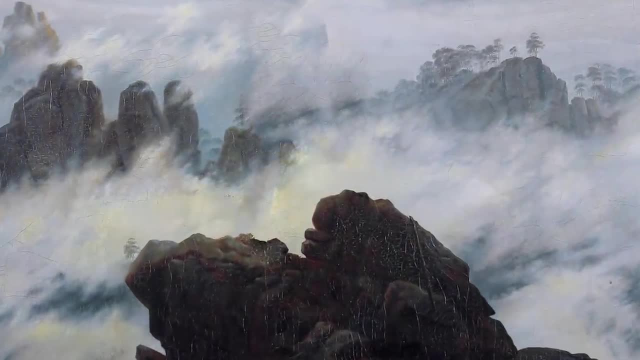 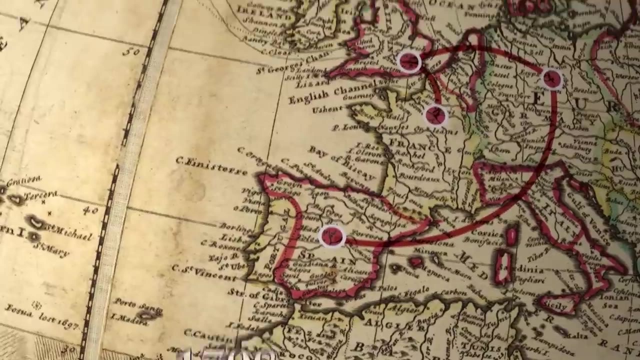 For a romantic, it's always right and noble to follow your heart. The disastrous results that follow aren't any argument. they're just proof of how desiccated and hard-hearted the so-called adult, sensible world can be. Madrid, Spain, 1798.. The artist Francisco Goya produces one of his most iconic images. 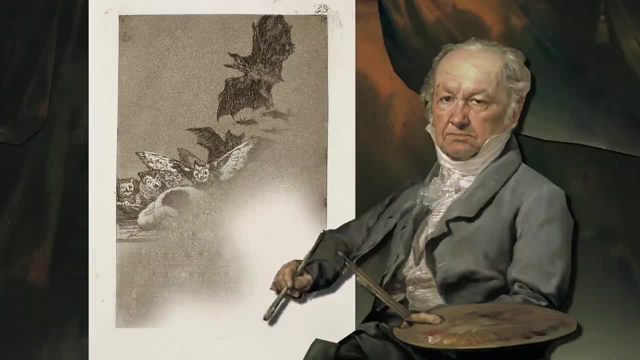 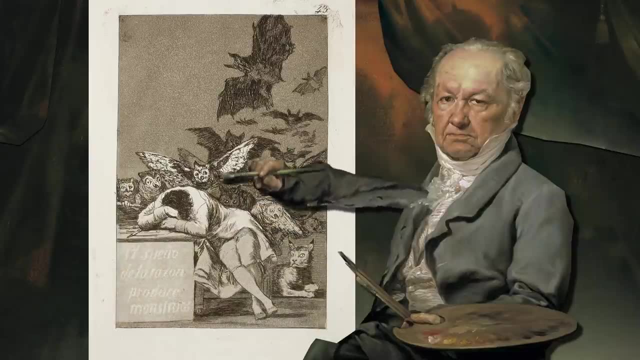 titled The Sleep of Reason Brings Out Monsters, It captures a quintessential romantic interest in the limits of reason and the power of the irrational over humans' fragile minds. To be romantic is to have sympathy for madness and to hold an almost vengeful attitude towards. 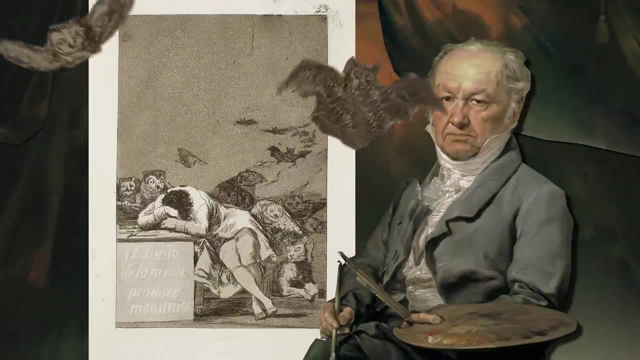 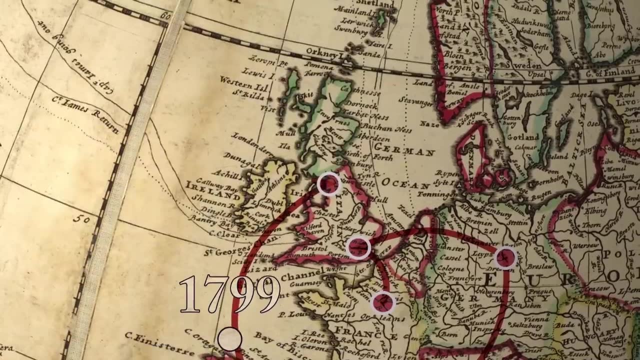 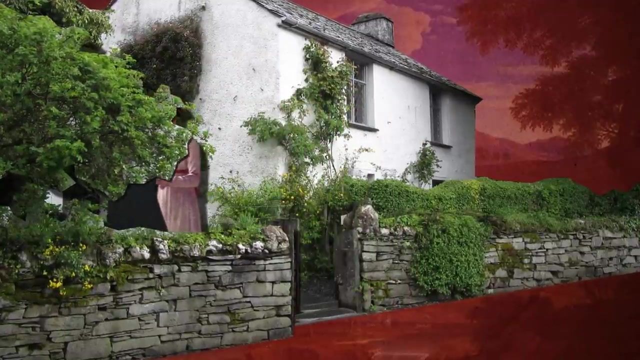 bombastic claims as to the true meaning of love. The lake district, England, December 1799.. A young English poet called William Wordsworth and his sister Dorothy move into what's set to become one of the most famous residences in the history of English literature – Dove Cottage in Grasmere, on the edge of the lake. 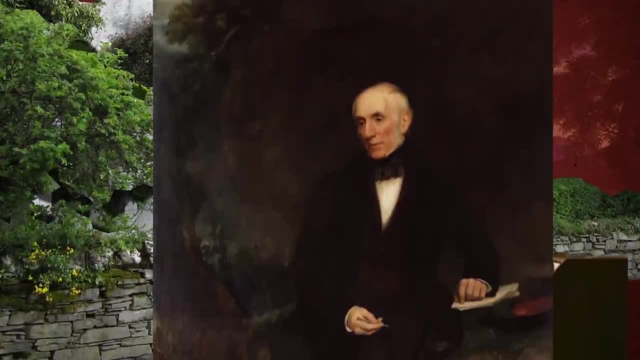 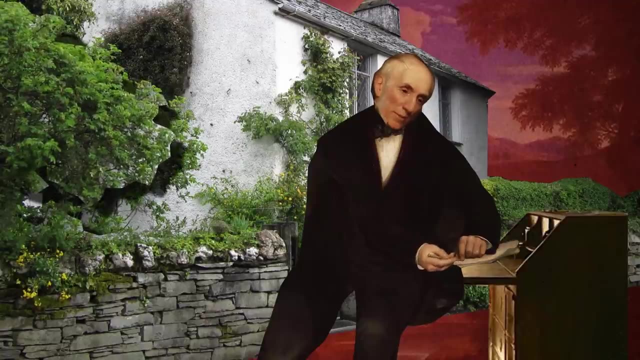 district. Here they will spend the next nine years, and Wordsworth will write some of the greatest poetry in the English language, celebrating something that's very under threat – the natural world. He'll write about daffodils, oak trees, clouds, butterflies and rivers, and his work. 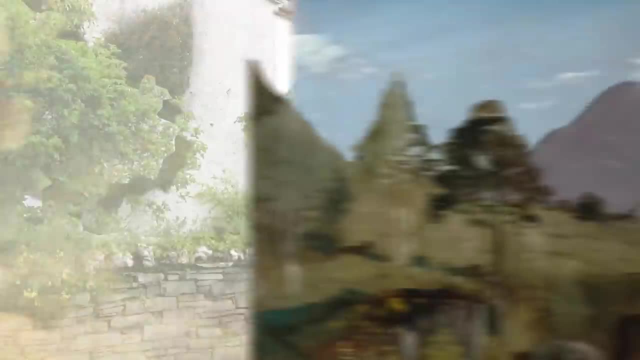 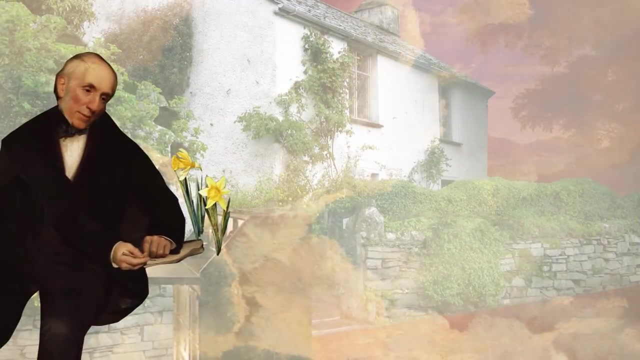 will charm and seduce Europe. Within a generation there will, in Wordsworth's own estimation, be more tourists than sheep in the lake district. Most importantly, running through Wordsworth's poetry is an abiding hatred for everything mechanical and industrial. When many years 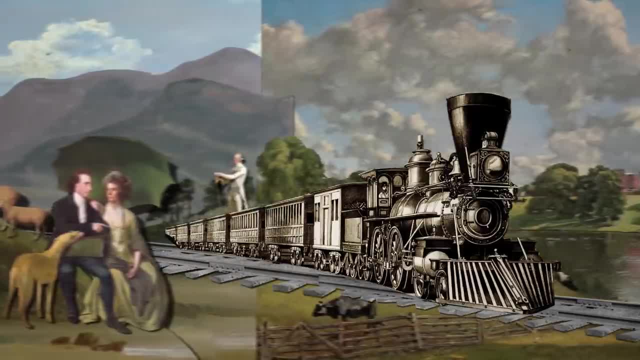 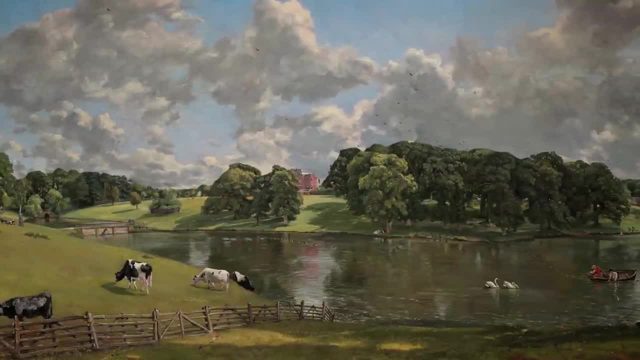 later, a railway line threatens to pass through the lake district. Wordsworth and his followers do everything they can to have the train- a symbol of Wordsworth's hated technology- be rooted. To be a Romantic is to take the side of nature against industry. It's to prefer a daffodil. 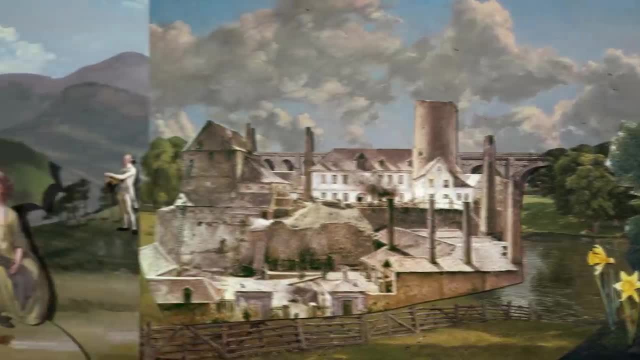 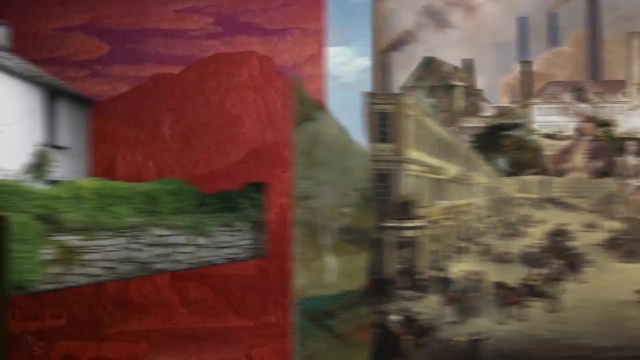 to a viaduct, a tree to a factory, At the moment when huge swathes of Britain are being covered in the often monstrous new cities that are making Europe rich, Wordsworth, the quintessential Romantic, speaks up for the natural and the simple life. 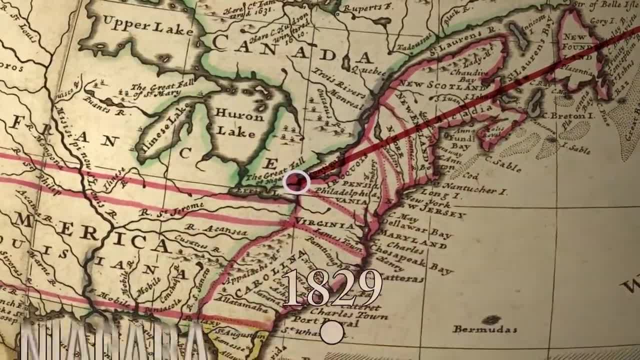 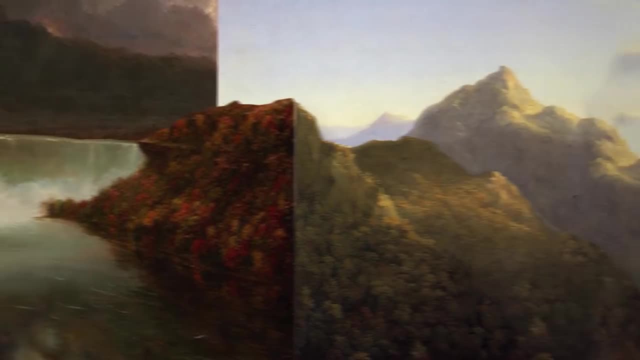 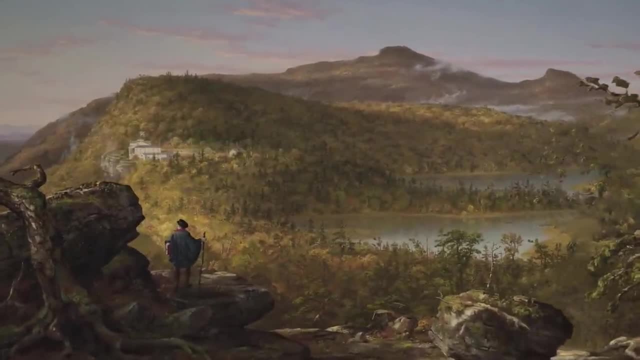 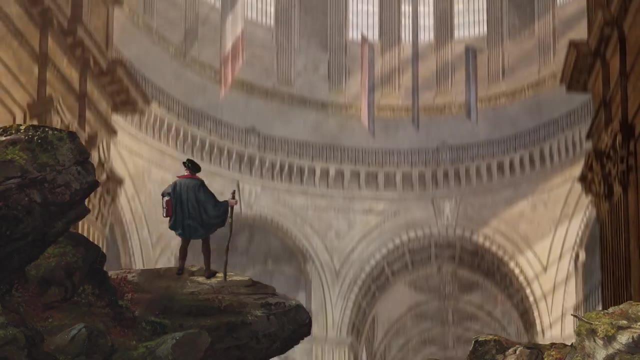 showing nature at its most dignified and impressive. Man looks lost and puny by comparison. This, too, is a typical Romantic attitude, for Romantics don't believe in God, but they go in search of the emotions one might once have had around religion and locate them in the big wide. 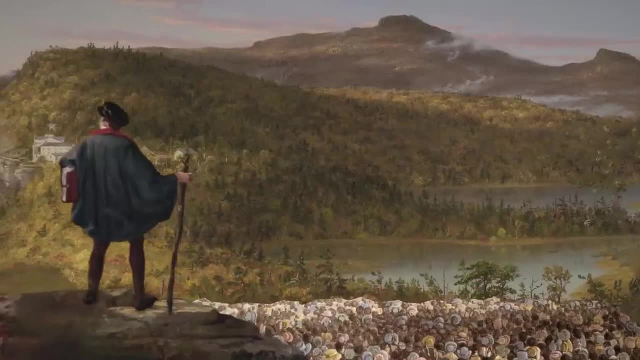 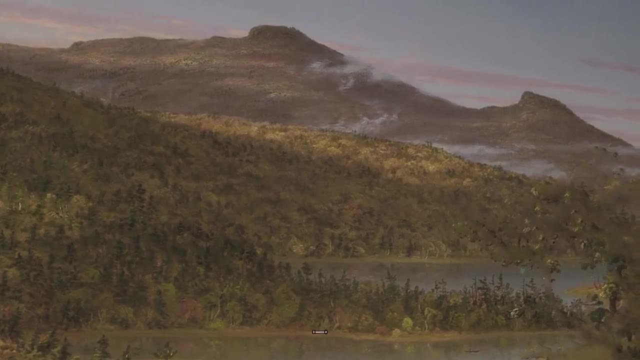 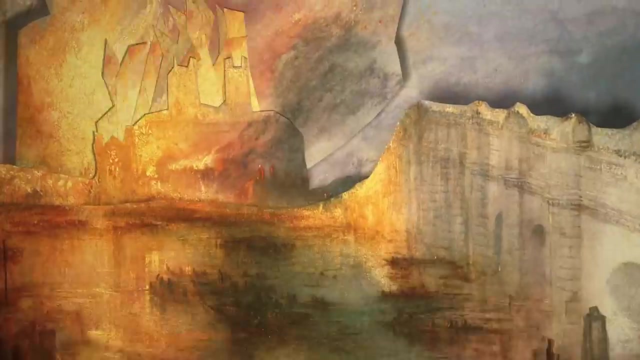 open spaces of nature. To be a Romantic is to find relief from the pressures of competitive city life in the sort of natural grandeur that transcends all human achievements and concerns Westminster, London, April 1847.. Fourteen years after some fairly incompetent officials, 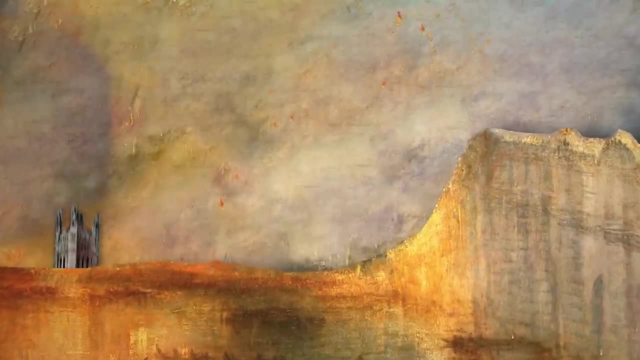 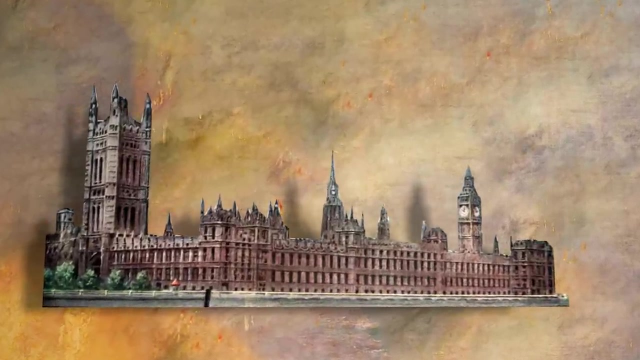 destroy the British Parliament with fire, a new building reopens, designed by a rising star architect, Augustus Pugin. Oddly, even though the building is new, it's made to look old, very, very old, medieval. in fact, It's full of suits of armour and seated angels. 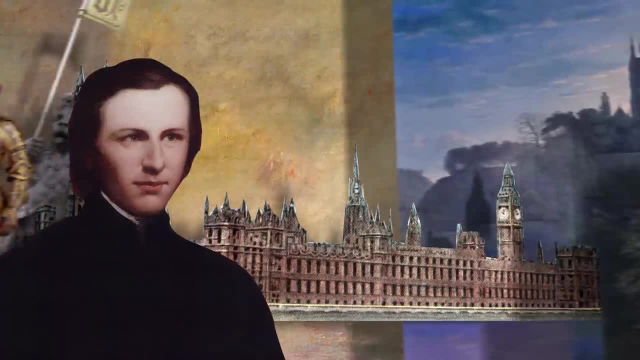 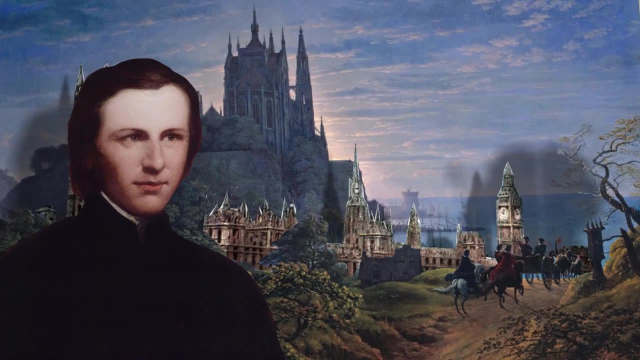 When the architect Pugin defends the building, he argues that his building is noble because it harks back to his country's pre-industrial past, before it grew obsessed, he's careful to add, with money or technology, It begins a cult of the Middle Ages, a big theme in 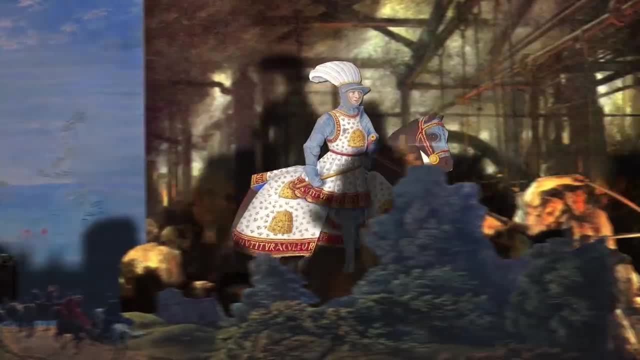 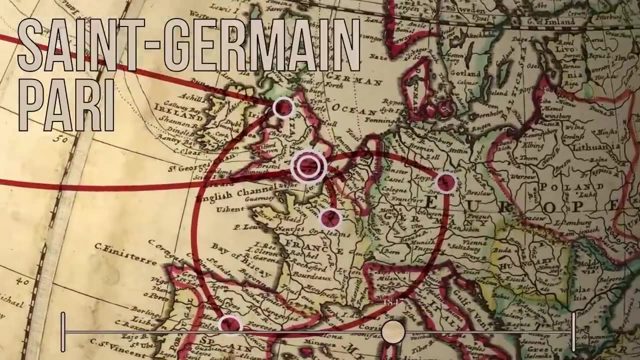 Romanticism, which identifies in the world of knights and castles, a nobility that is thought missing from the factories and shopping arcades of the modern world. Saint-Germain, Paris, May 1863.. The French poet Charles Baudelaire writes a prose poem.